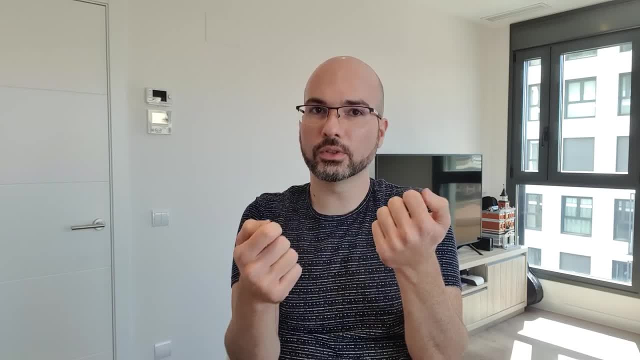 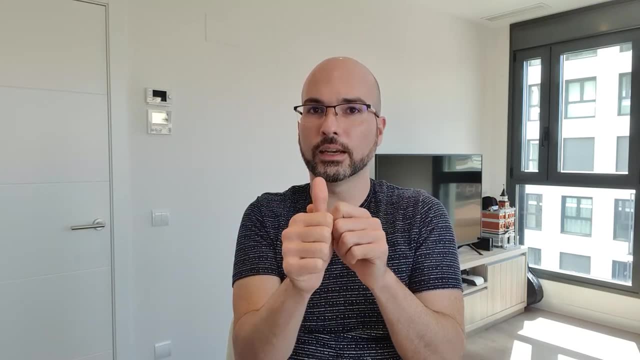 catching the results of some problems, and there are two conditions to be met in order to know if a problem is a good fit for using dynamic programming. Basically, one is having an optimal substructure. That means that the optimal solution can be constructed for finding the 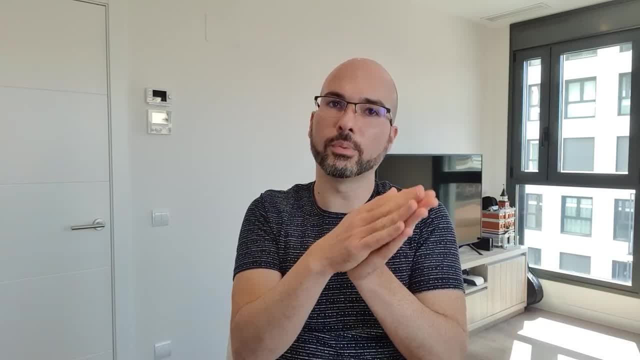 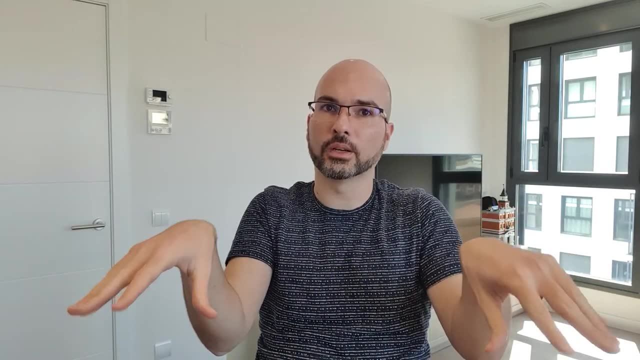 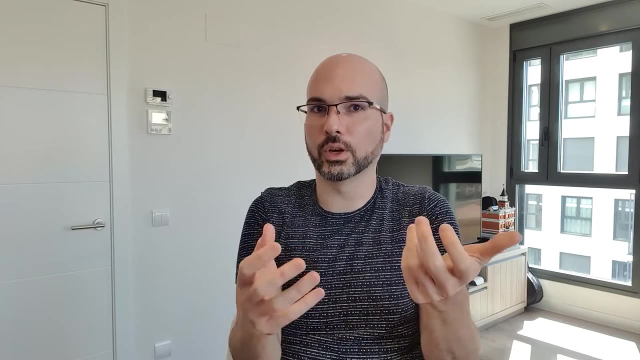 optimal solutions of itself problems and that they are overlapping some problems. So, for example, Mershford is not a good candidate for dynamic programming because you have two different sets of problems to solve. It's not. you're not having overlapping some problems. I will now show you a little bit of an example, using the most common example. 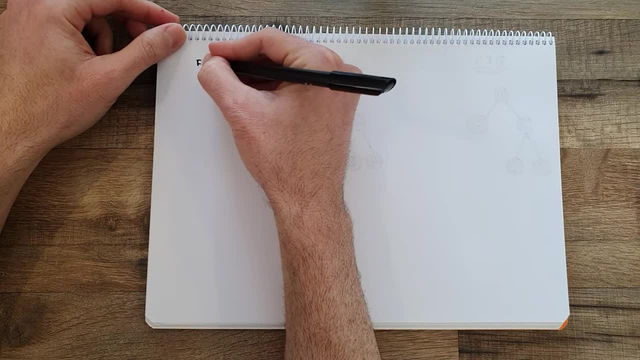 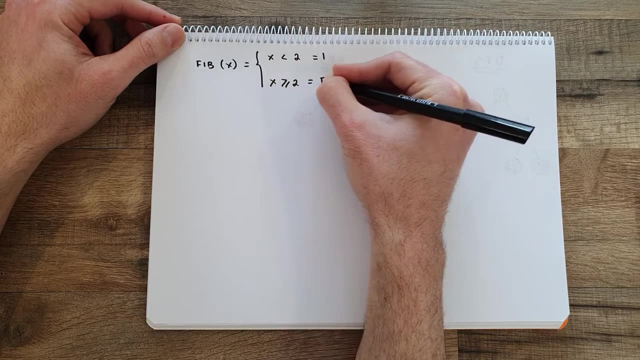 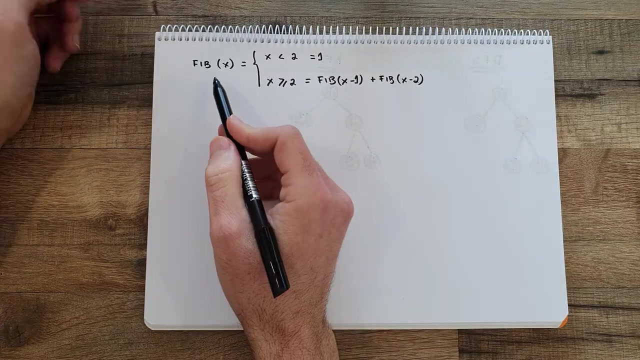 for recursion, that is a fibonacci. So here we see the definition of the fibonacci function, right? So fibonacci of a number, x would be. if x is less than two, it would be one. If x is equal or larger than two, then it would be fibonacci of x minus one, plus fibonacci of 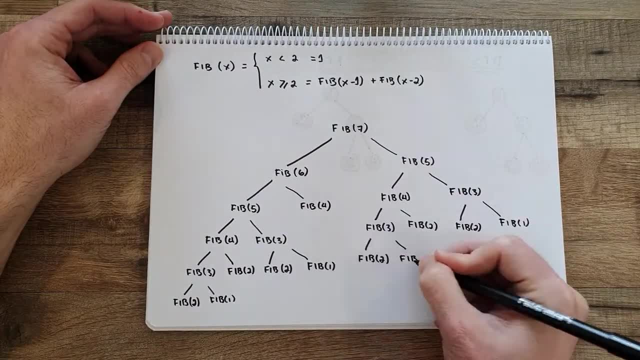 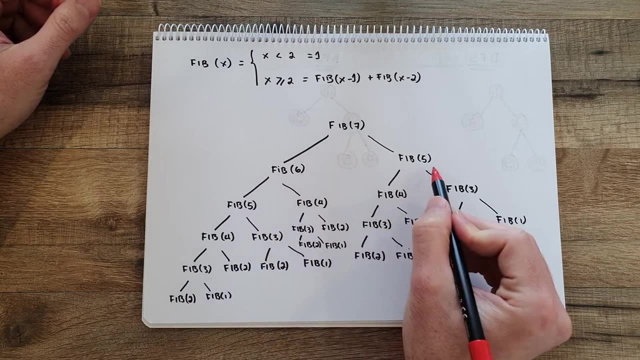 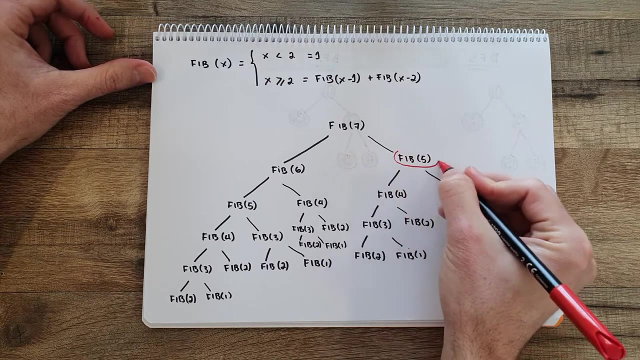 x-2.. Let's say we want to calculate Fibonacci of 7.. If you see down the tree, we will see that we need to calculate Fibonacci of 6 and Fibonacci of 5, which is getting duplicated in different parts. right, So we can see that Fibonacci of 5,, for example, is calculated. 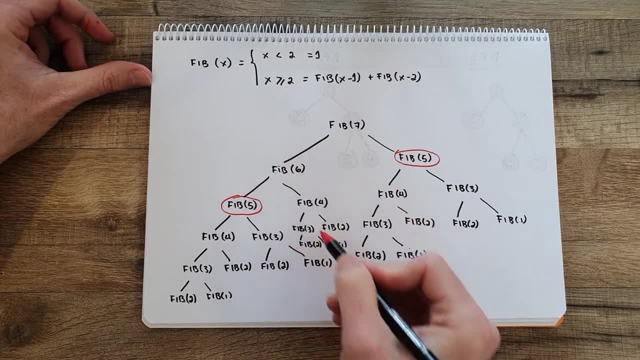 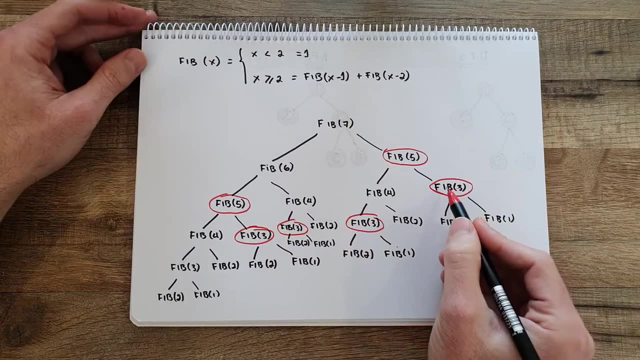 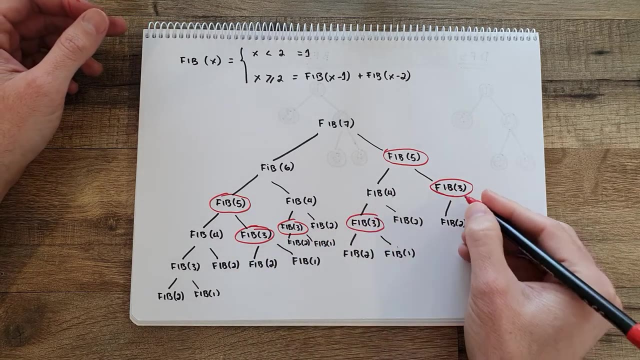 here and here And if we go more into the tree, we also see more duplication, like Fibonacci of 3,, for example, being calculated in different times. So you can see that once Fibonacci of 3 is calculated, all of the other Fibonacci of 3 are the same basically. So they are. 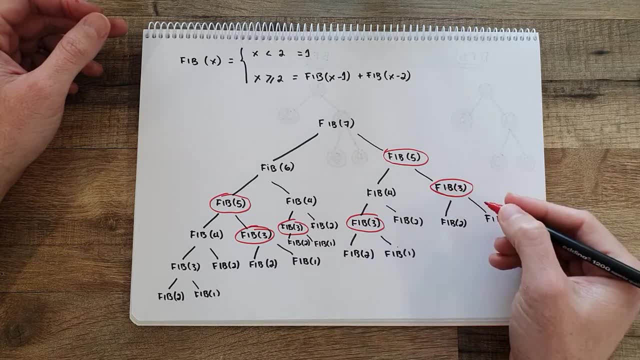 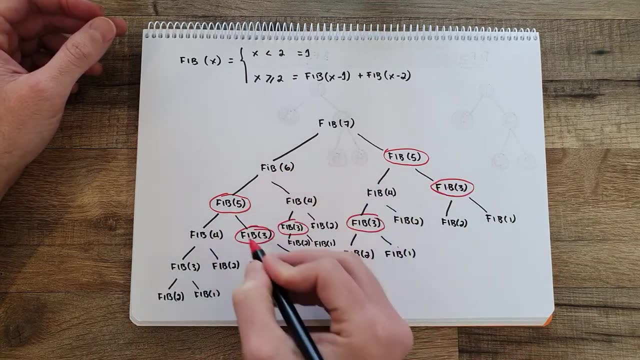 like, calculated at once, it would be already the optimal solution, And we can see that each of the problems are overlapping with each other, right? So you have Fibonacci of 5 getting overlapped here and Fibonacci of 3,, 4, etc. right? So this is a good example. 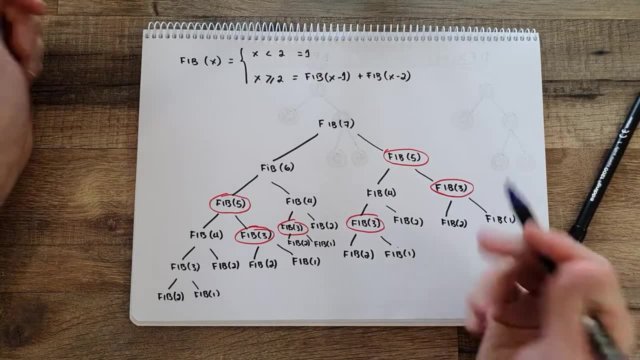 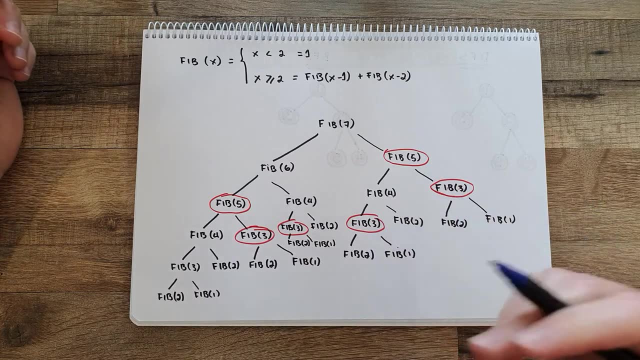 of why dynamic programming can be useful to solve this problem. So what you would do in dynamic programming is to catch these solutions, these subsolutions, into a data structure that you can use Later to avoid recalculating them. So, for example, if you are calculating the whole, 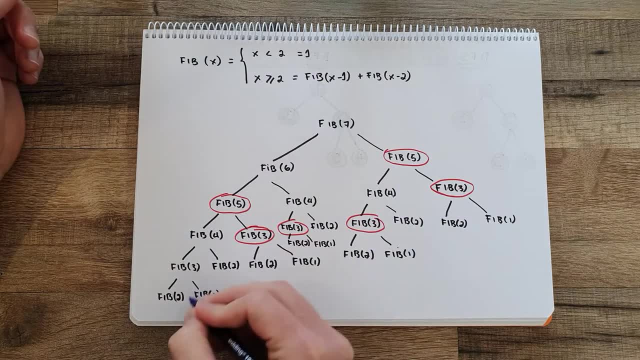 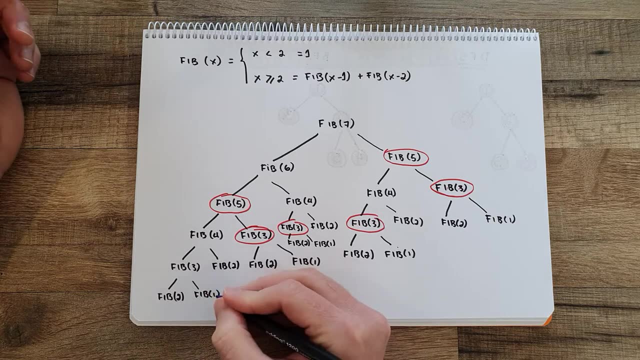 tree, you need to start with Fibonacci of 1, right? And if you're starting with this branch here, let's say it's the first time that you encounter Fibonacci of 1.. So you would say: okay, so it's not calculated, I will store Fibonacci of 1 to be 1.. And then 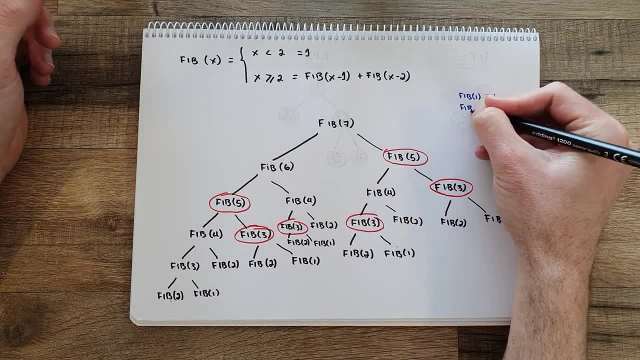 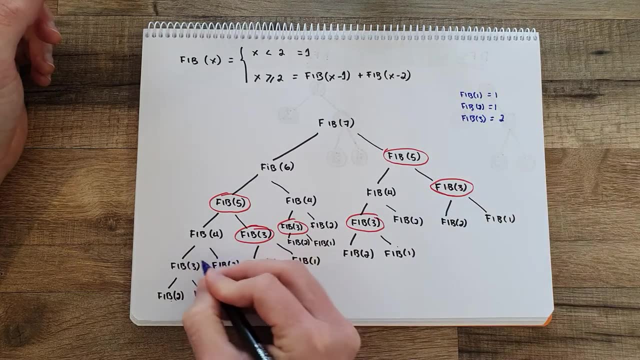 you go to Fibonacci of 2, and will be Fibonacci of 2, will be 1 as well. And then you go to Fibonacci of 3, and Fibonacci of 3 will be then be 2.. Then you go to Fibonacci of 4,, but you already know like did I calculate Fibonacci of 2?? Yes, 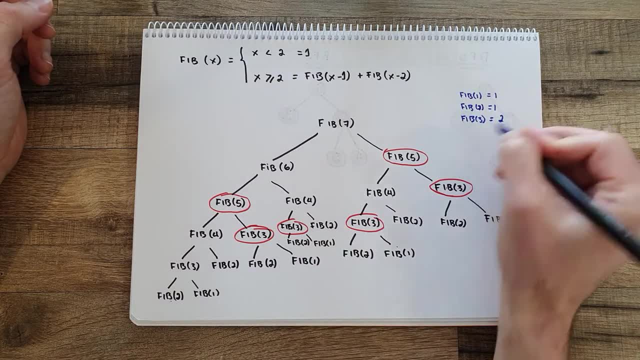 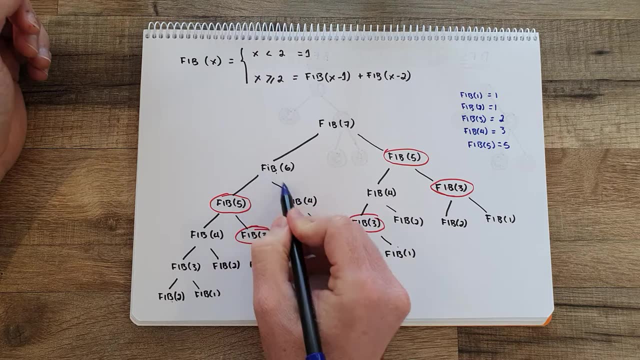 I calculated Fibonacci of 2.. And then I also calculated Fibonacci of 3,, so I can calculate Fibonacci of 4, and so forth, so on. So what you do then is, when you go here, for example, Fibonacci of 6,, instead of calculating again the whole tree, what you do is: what is Fibonacci? 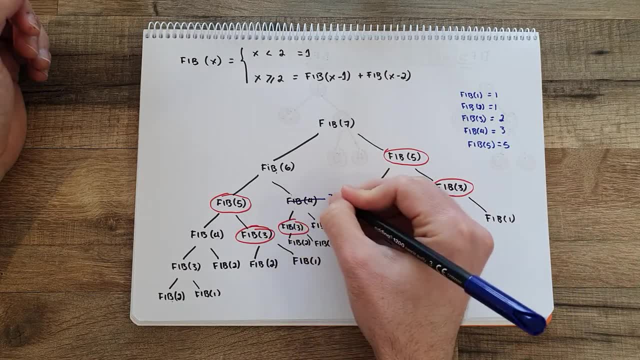 of 4? So you will know that Fibonacci of 4 is 3, so you just replace this with 3.. You don't need to calculate the whole tree, right? So you save a lot of computation time here instead of doing the whole recursion. 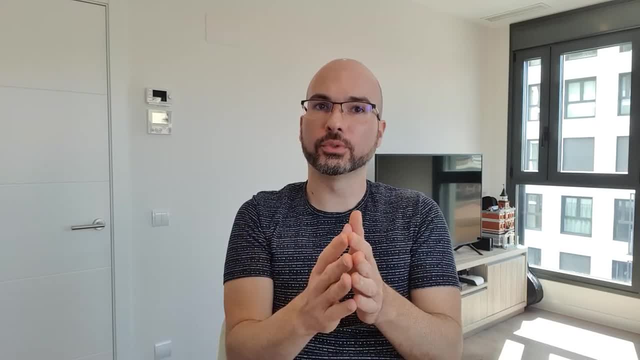 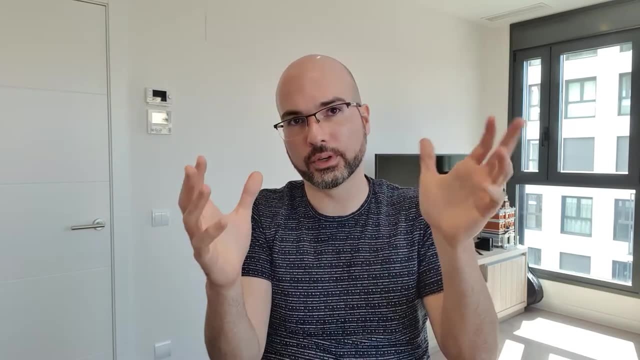 So recursion and dynamic programming are very useful tools and you can use them whenever you find the need for it. Some problems might be easier to approach when you are thinking about them recursively. Of course, recursion also has some impact on the memory, so if 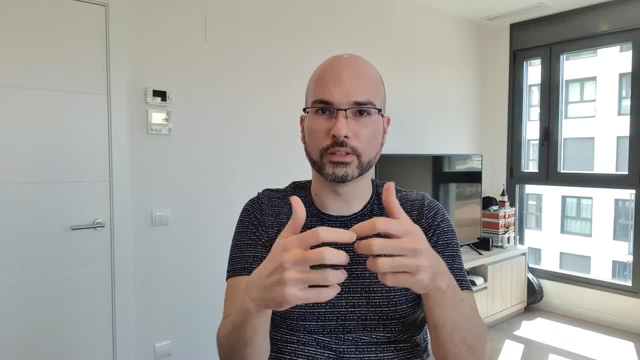 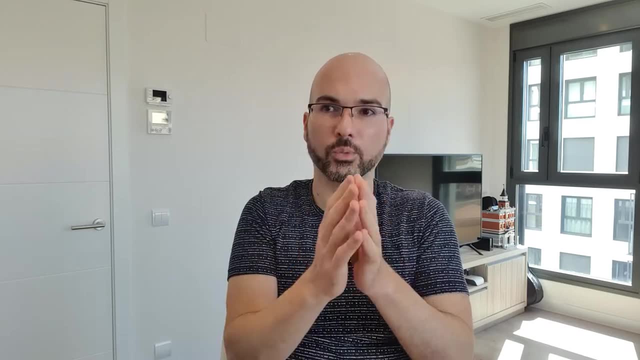 you're looking for the most efficient solution or you're trying to optimize a problem that you solve using recursion, it's usually better to convert it into an iteratively solution. One of the most easiest ways to do it is by using what is called tail: recursion and tail. 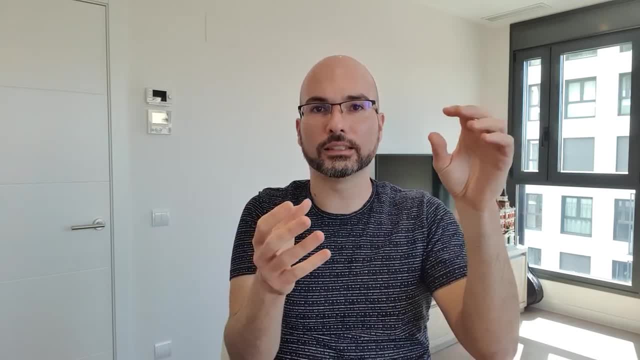 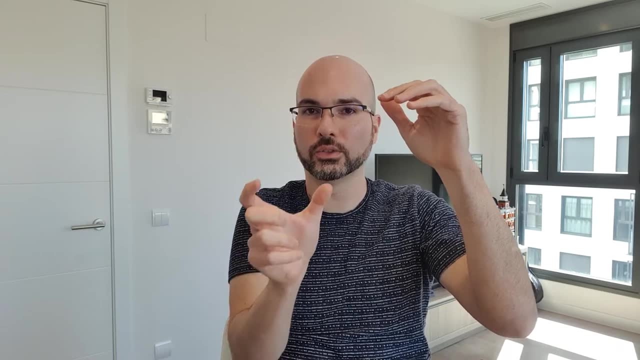 recursion. So basically what tail recursion means is it's a function where you have all your block of code and you do all the computation and at the end you call your recursive function and you don't do anything else after that. And many languages are able to even optimize. 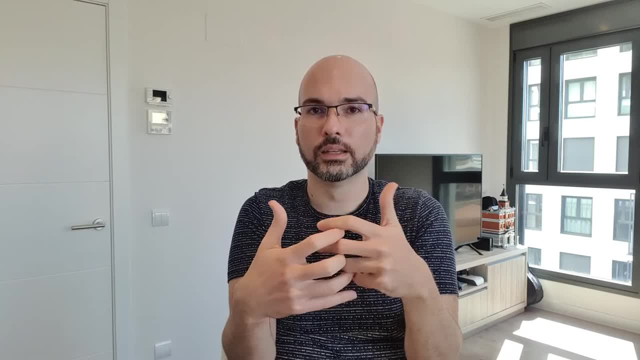 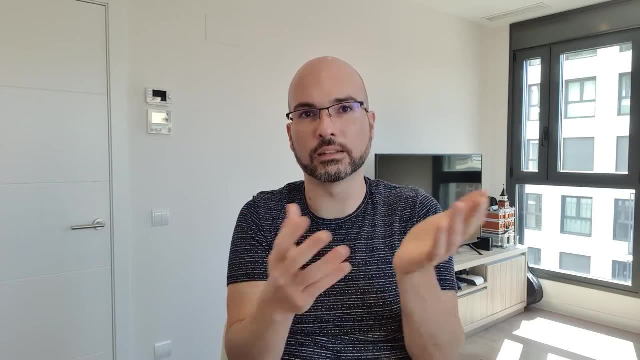 tail recursions into iteratively at runtime, But you can convert. once you have a tail recursion, it's more easy to convert it into an iteratively solution. So that's it about recursion and dynamic programming, and if you want me to explain a little bit more, or 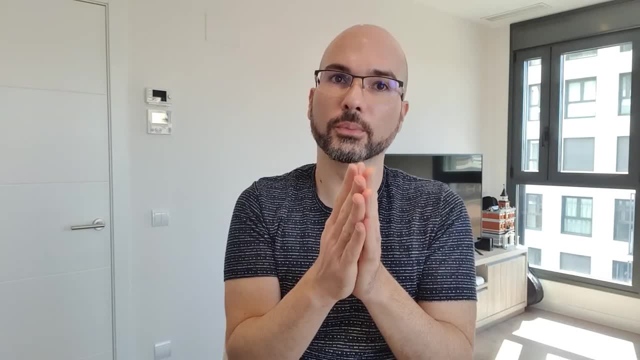 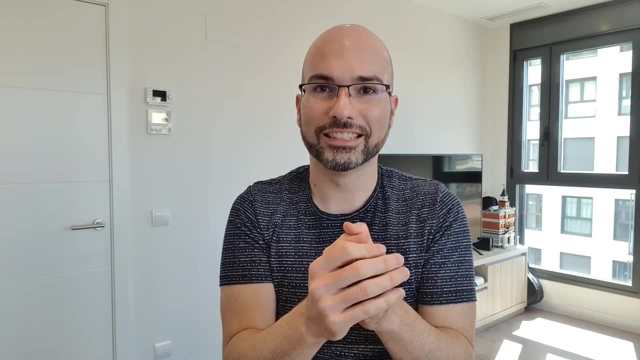 have more examples, just don't forget to comment there. I also put some links in the description And, of course, if you liked the video, just don't forget to like it, subscribe, share it with your friends and that's it. Thank you for watching. See you next time.